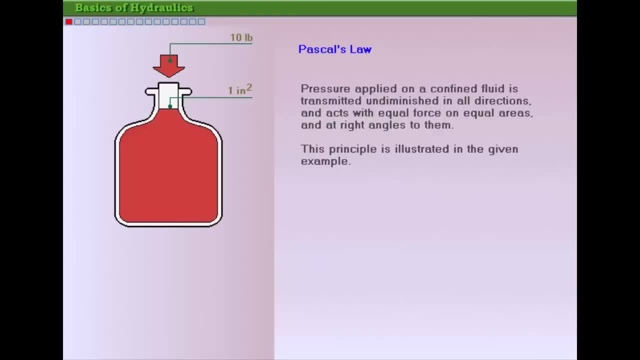 times area. Pascal's law states that pressure created in a confined fluid is transmitted undiminished in all directions. How does Pascal's law work? The following example of a glass bottle filled with fluid clearly illustrates Pascal's law. A small input force is applied to the stopper Pressure. 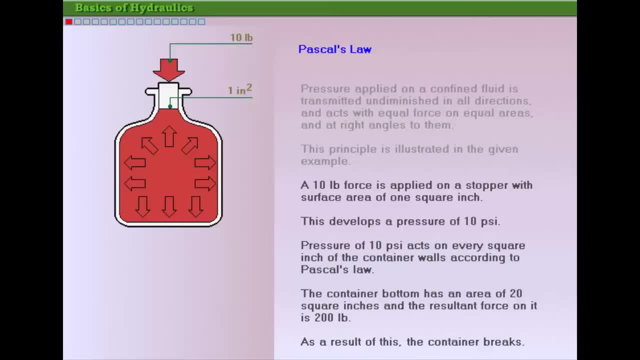 equal to the force divided by the stopper area is created in the fluid. In this case, it is 10 pounds per square inch of pressure, as we have applied 10 pounds of input force over an area of 1 square inch. According to Pascal's law, this pressure is then transmitted. 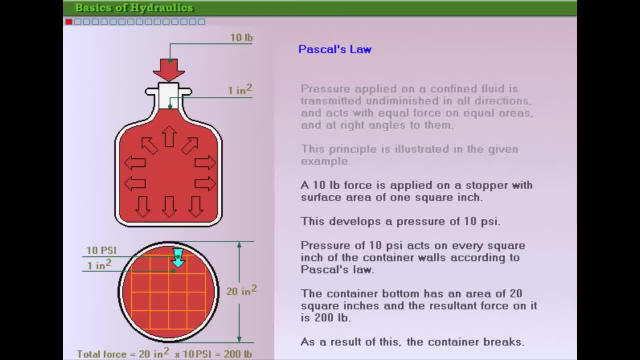 through the fluid undiminished in all directions. This pressure acts against all equal areas of the bottle. The resultant output force is multiplied, in this example, over the 20 square inches of the bottom of the bottle. In this case, an output force of 200 pounds. 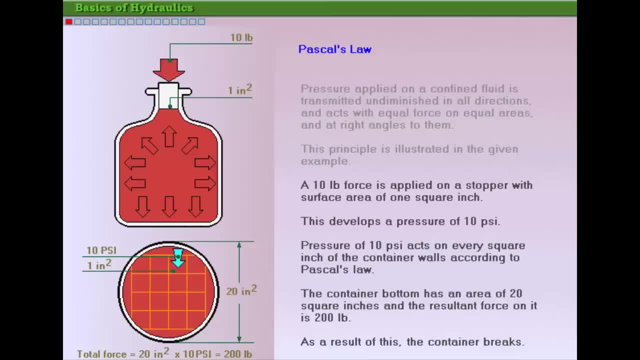 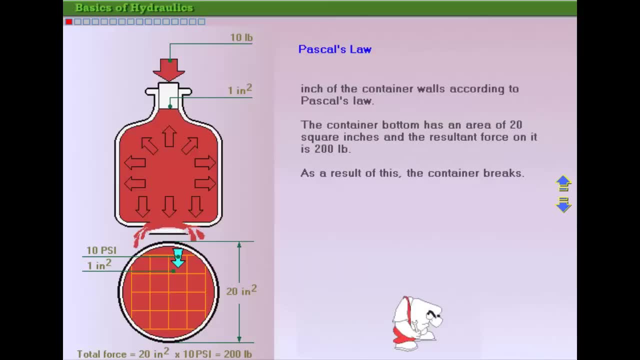 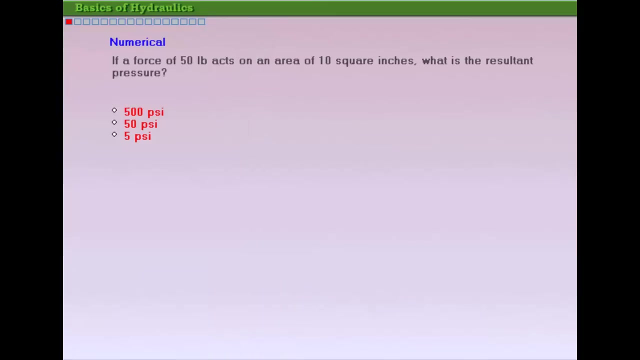 is generated with an input force of only 10 pounds. Due to this increased force on the bottom, the bottle breaks. What will be the value of pressure developed if a force of 50 pounds acts on an area of 10 square inches? 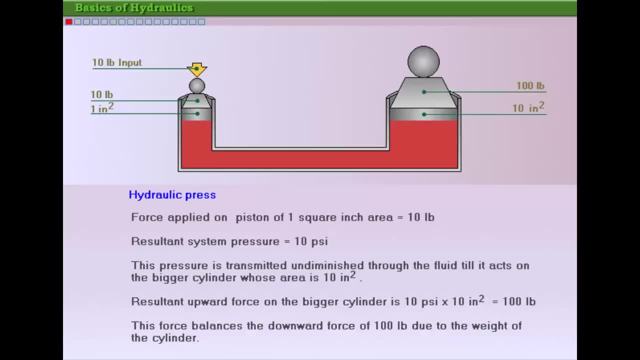 The hydraulic press uses the principle stated in Pascal's law to multiply force applied on a small area to a bigger force from a larger area. Let's see how Brahma, a British mechanic, applied Pascal's principle to the hydraulic press. A force of 10 pounds is applied to a piston area equal to 1 square inch. 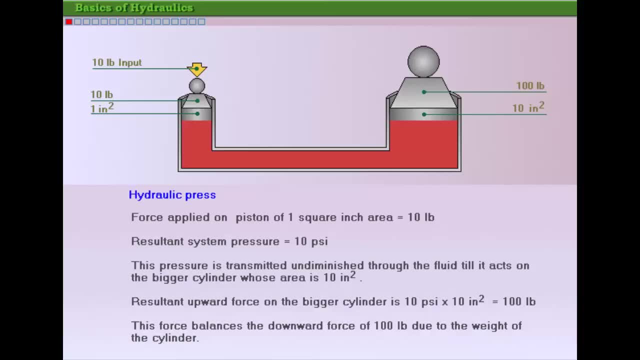 The resultant system pressure is then 10 pounds per square inch or 10 psi. This pressure is transmitted undiminished through the fluid and acts on the bigger cylinder whose area is 10 square inches. The resultant upward force on the bigger cylinder is 100 pounds.